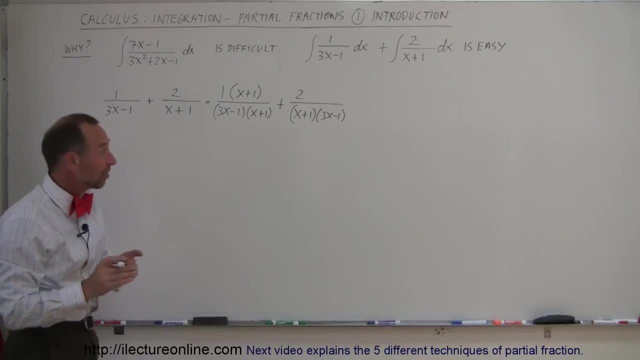 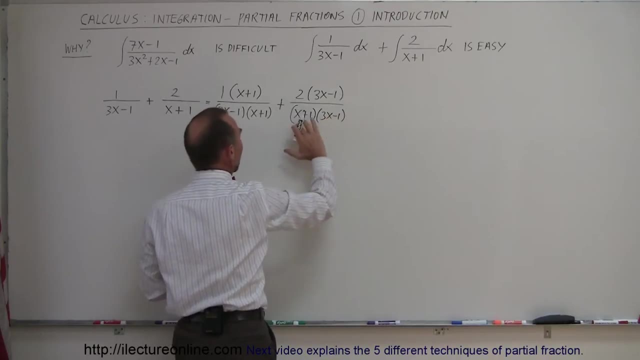 multiply the denominator by 3x minus 1. I have to do exactly the same to the numerator. I also have to multiply it by 3x minus 1.. Notice, when I cancel these two out I get back what I started with right here. but now I realize that those 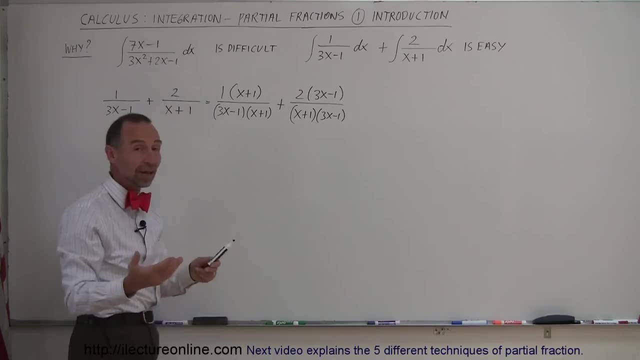 two fractions should be actually 1 over 3x minus 1 and I have to do exactly the same fractions have the same common denominator, so I can write them over the same denominator, so I can say: well, this is equal to well, 1 times x plus 1 is 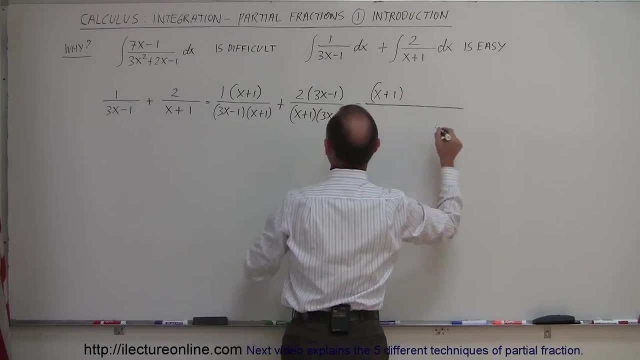 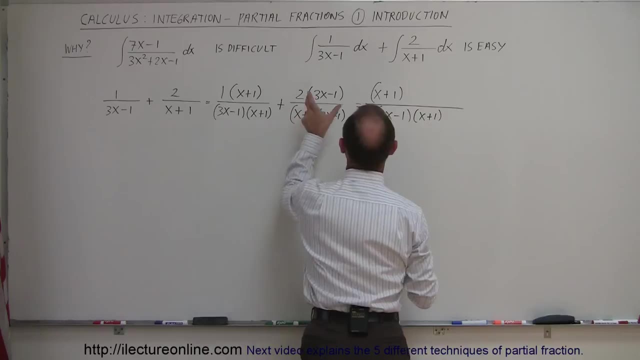 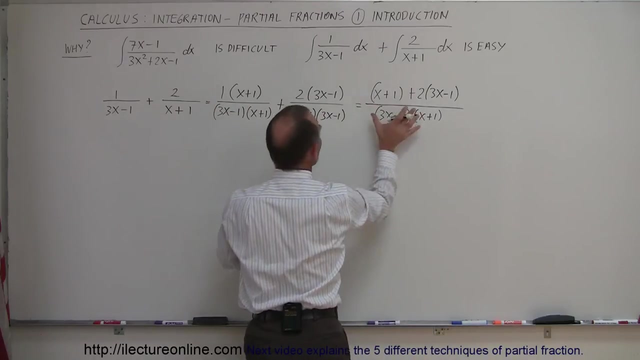 simply x plus 1 divided by 3x minus 1 times x plus 1, right there. and then I add to that this one right here, which we have 2 times 3x minus 1. so now I simply wrote them over the same common denominator. now I simplify that by: 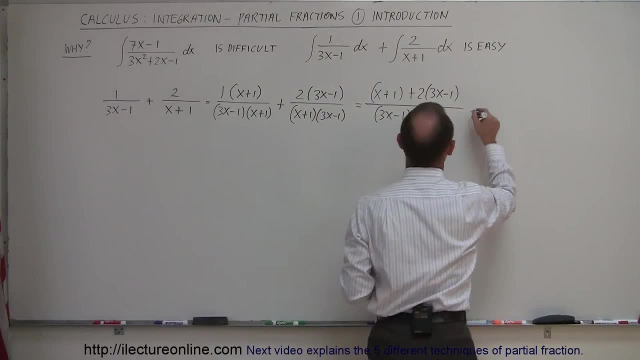 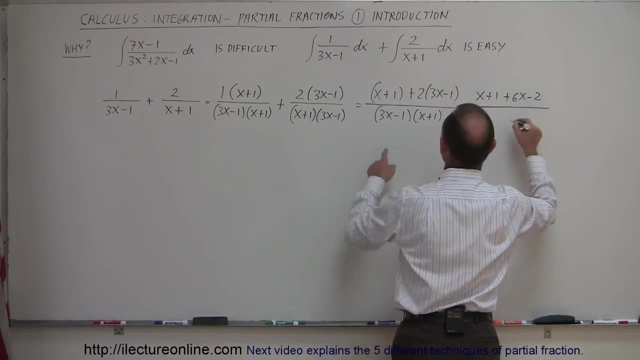 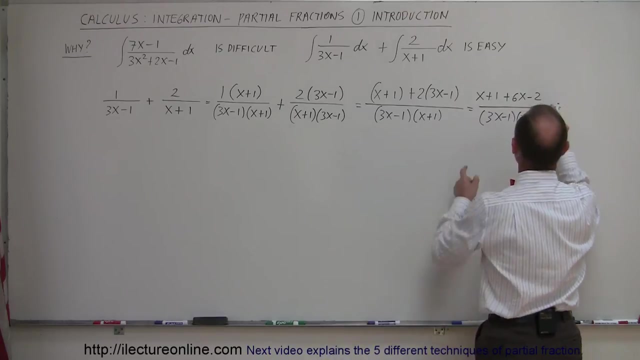 getting rid of the parentheses and adding common common terms. so this is equal to x plus 1 plus 6x minus 2, all divided by 3x minus 1, divided by and times x plus 1. all right, and I'm collecting common terms. x plus 6x is 7x. 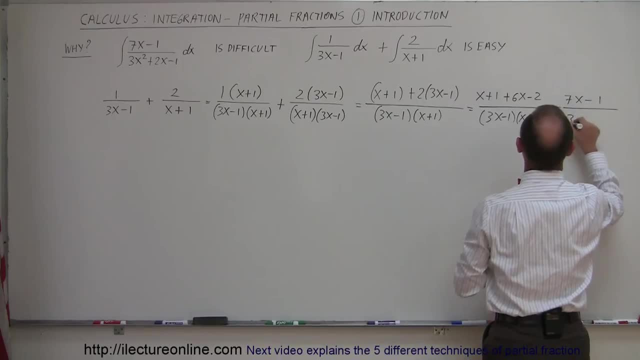 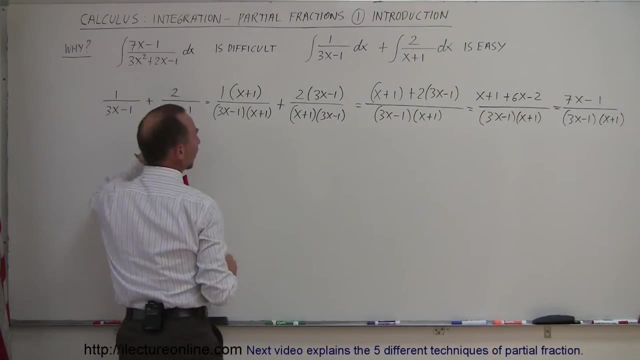 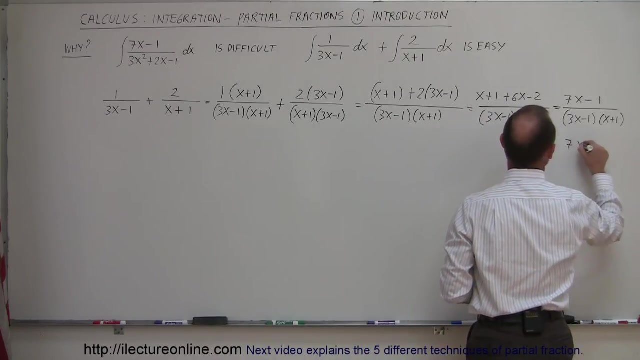 and 1 minus 2 is minus 1 divided by 3x minus 1 times x plus 1. so now notice what you have over here looks exactly the same as well. not exactly the same. yet let me go. let me multiply out the denominator. so we have 7x minus 1 3x times x is 3x squared 3x. 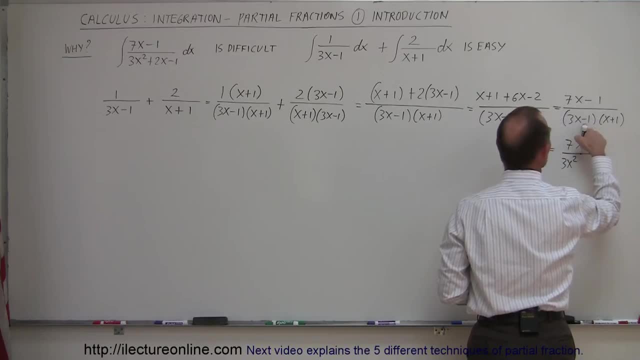 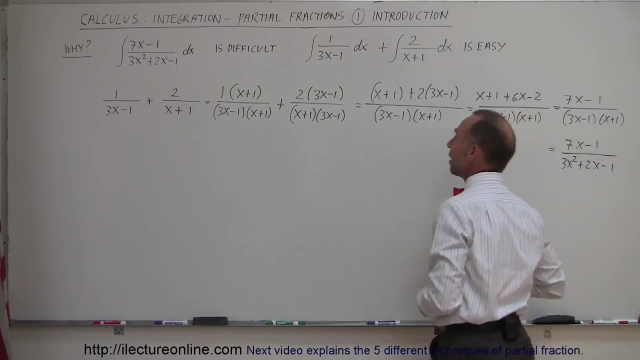 times plus 1 is 3x, x times a minus 1 is minus x. so 3x minus x is plus 2x, and minus 1 times a plus 1 is minus 1. do they look the same now? yes, now they do. 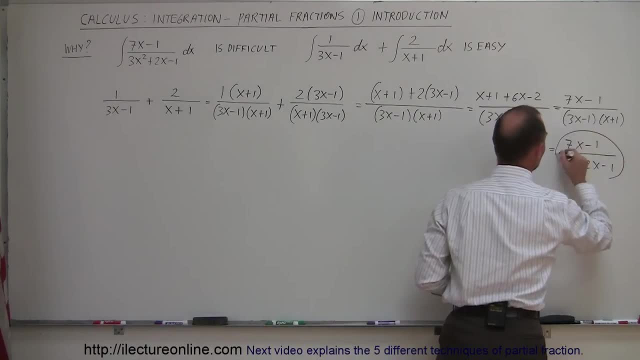 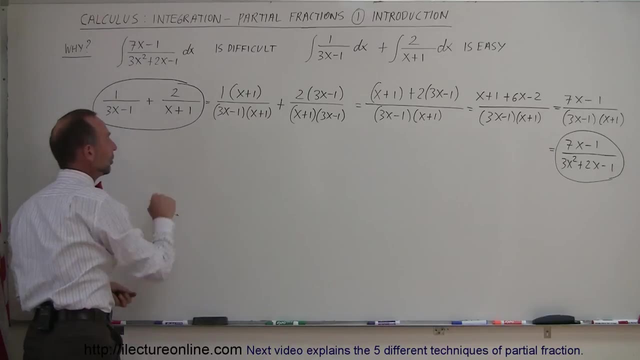 all right. so notice that this right here is exactly the same as those two fractions added together right here now, since I can easily integrate those two and I can integrate this one, the trick is to take something that looks like this: if it doesn't need an integral sign right here,